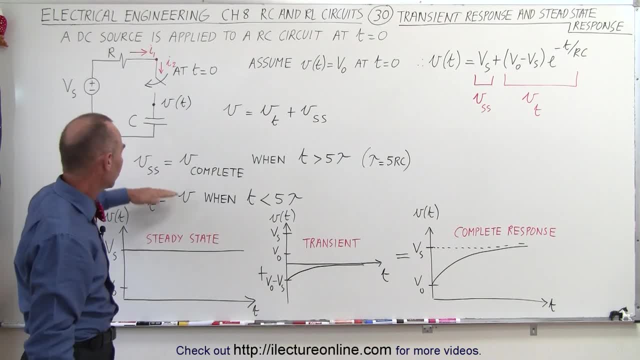 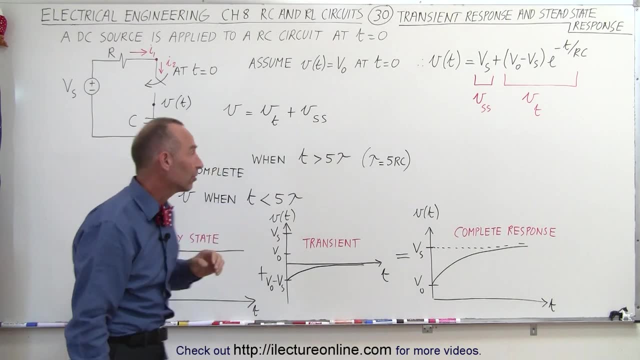 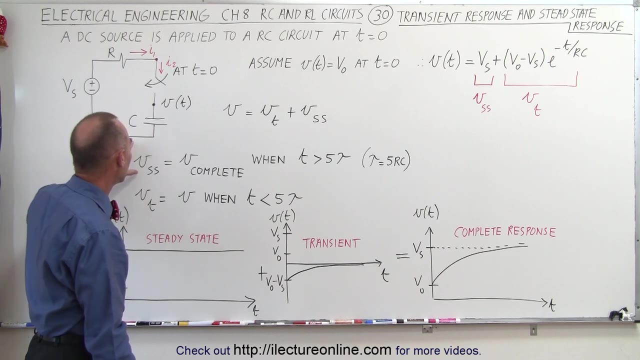 only active for the first five time constants of the circuit. So we could say that the steady state is equal to the complete response when the time is greater than five time constants. and when the time is less than five time constants we also have the transient response, which is added. 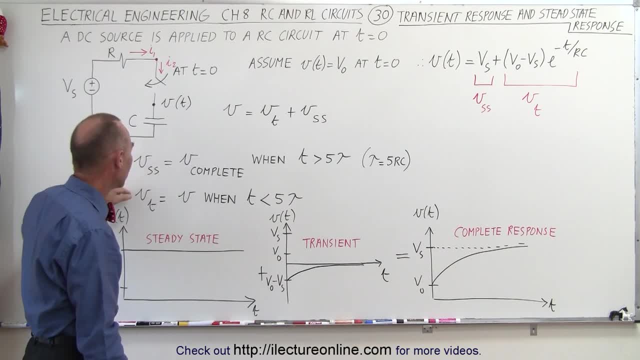 to the steady state response. So the two together is the response you get during the first five time. constants of the circuit. So if we then take a look at what the steady state looks like over a long period of time, the voltage across the, the voltage across the circuit, is equal to the steady state. 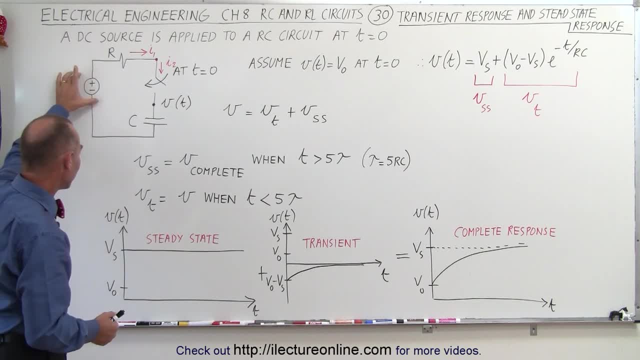 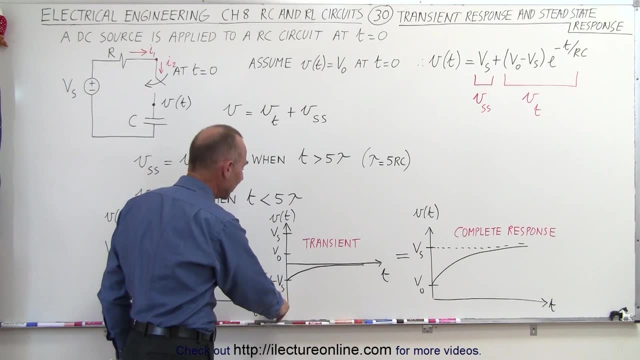 The capacitor will be equal to the voltage of the source. But during the transient state, notice that this is the response of the circuit, where we go from the point V minus V of the source- so that's negative voltage- until we get down to the zero voltage. So when we look at this portion of the 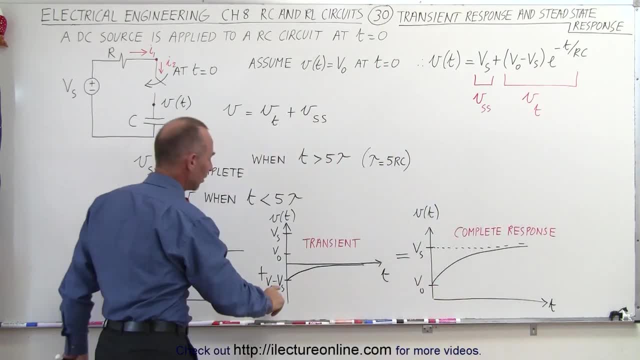 equation right there that represents a voltage that goes from V minus V via the source all the way to zero volts. That's the transient state. when we combine the two, then this is what the complete response of the circuit will look like, where the, where the voltage across the capacitor goes from. 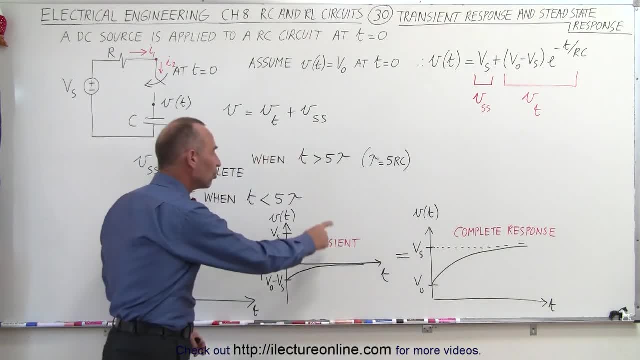 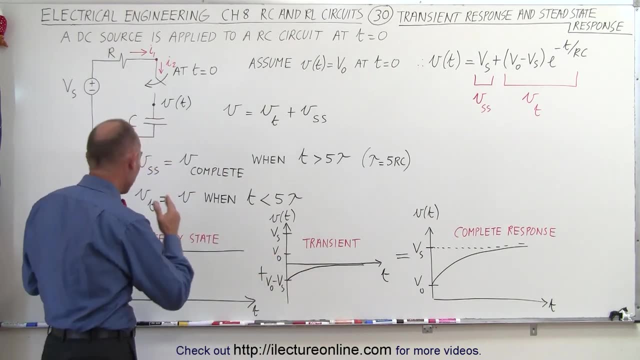 the initial voltage to the steady state voltage. So the transient is often misunderstood. it does indeed look like there's a negative voltage, but what happens is we apply. we apply the source to the circuit and until this the voltage across capacitor reaches the voltage of the source. 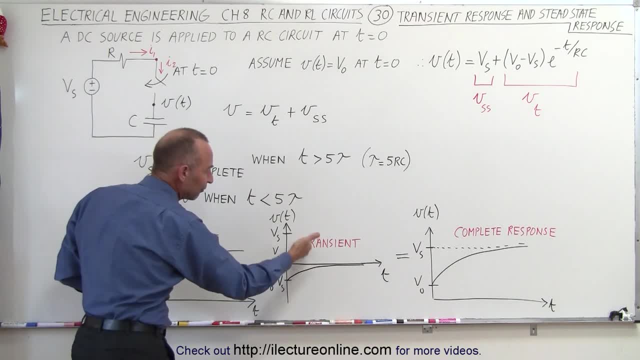 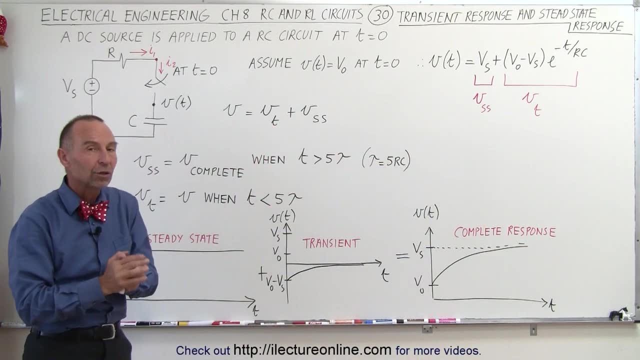 it's in essence: we take the steady state and we add a negative voltage to it that eventually goes to zero to get the real complete response of the circuit. So the transient state is only what happens to the circuit over a short period of time, namely the first five time constants. 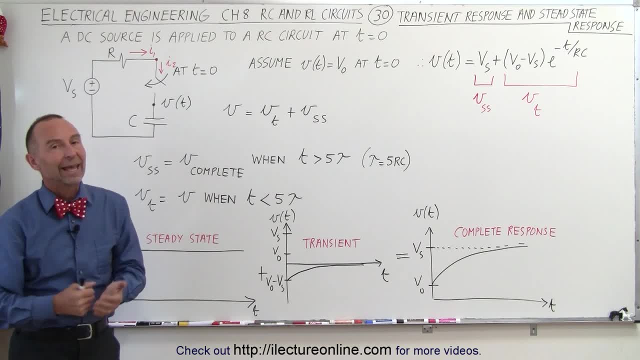 and that's what we mean by the difference between the transient response and the steady state response.